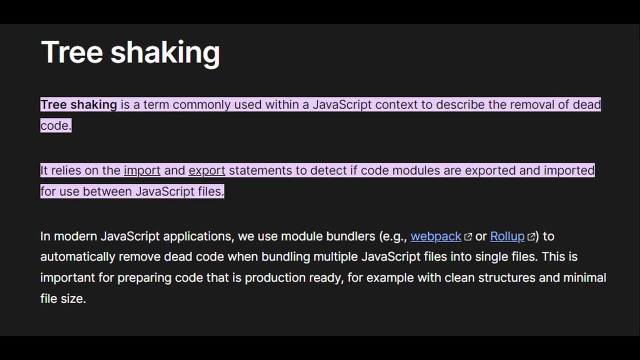 Tree shaking is a technique used by modern JavaScript bundlers such as Webpack or Rollup to eliminate dead code from the final bundle. Dead code refers to parts of your JavaScript codebase that are never executed or used in your application. The process of tree shaking. 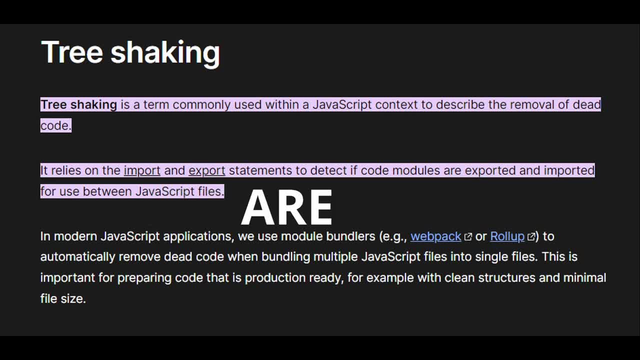 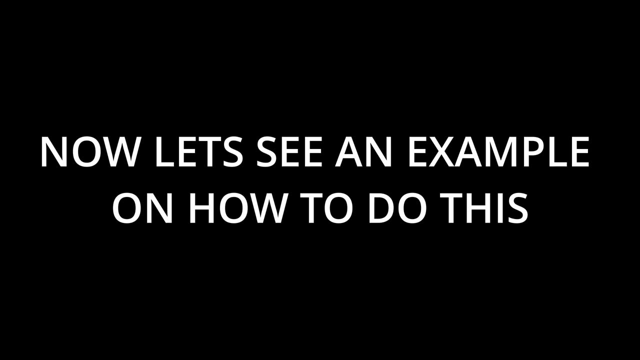 involves analyzing your codebase and identifying which parts are actually used and which parts are not. The unused parts are then removed from the final bundle, resulting in a smaller bundle size and improved performance. So how to enable tree shaking using Webpack to improve our application's performance. 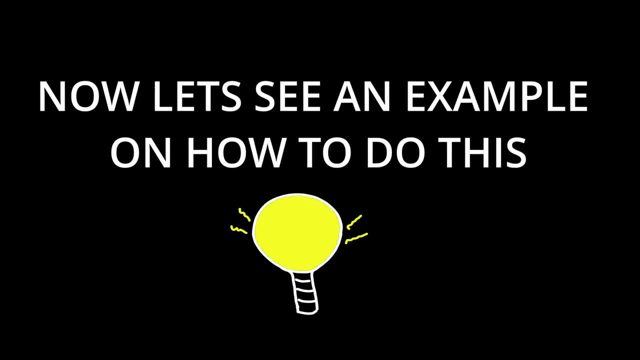 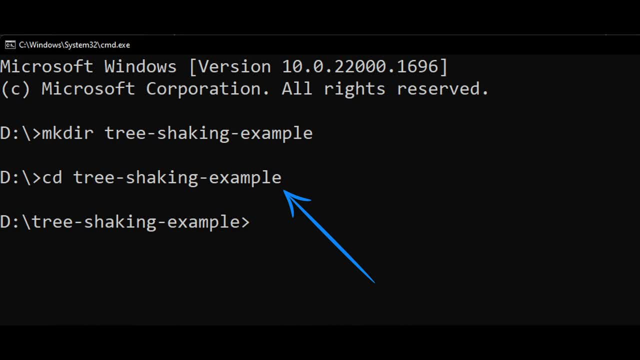 For that, let's see an example with some simple JavaScript code and minimal Webpack setup. First create a new directory for the project and navigate into it in your terminal. I will name my directory as Tree Shaking Example. Then initialize a simple new Nodejs. 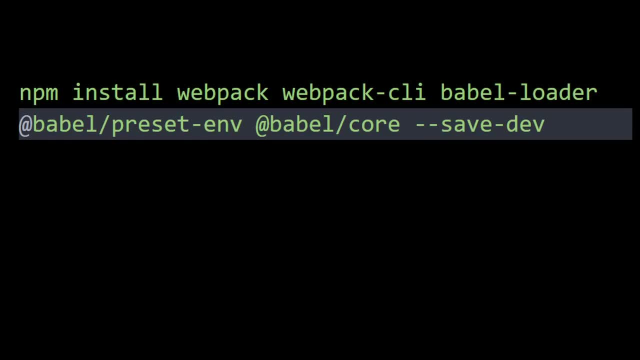 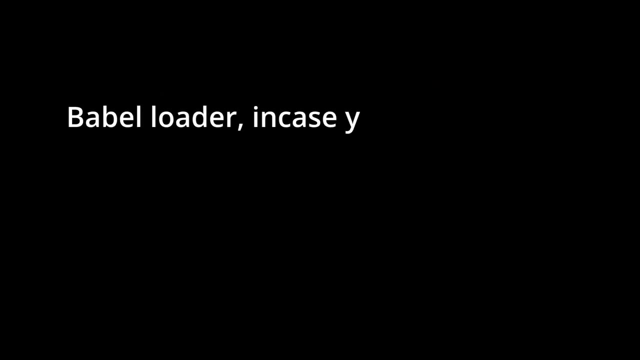 project with NPM in it. After that, install the required dependencies: Webpack, Webpack CLI, Babel Loader and Babel Preset Env. Babel Loader, in case you didn't know, is used to convert code written in modern JavaScript. 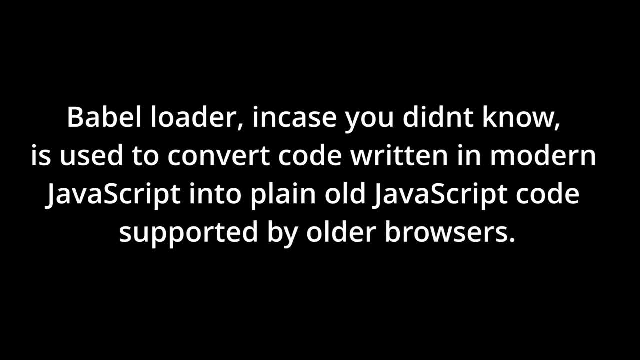 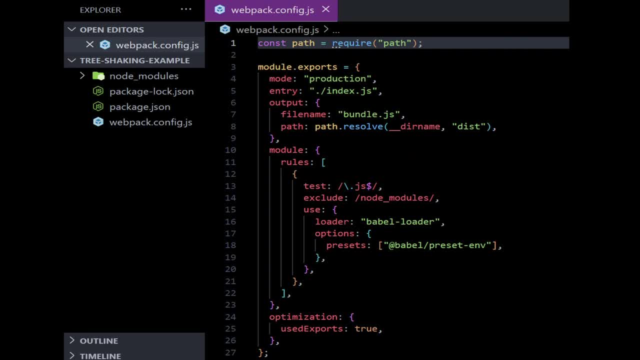 into plain old JavaScript code supported by older browsers. Then create a new file named webpackconfigjs in the root directory of your project with the following configuration: All this configuration does is it sets up Webpack to use Babel to transpile your JavaScript code and enables tree shaking by setting the used exports optimization. 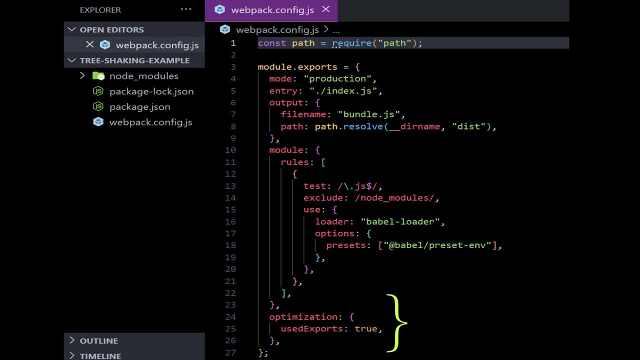 flag to true. This part, setting the used exports optimization to true, is what enables tree shaking, and it's all we are concerned about for this tutorial. If you want to know how to set up Webpack and what these other terms mean, then that's for a whole different tutorial. 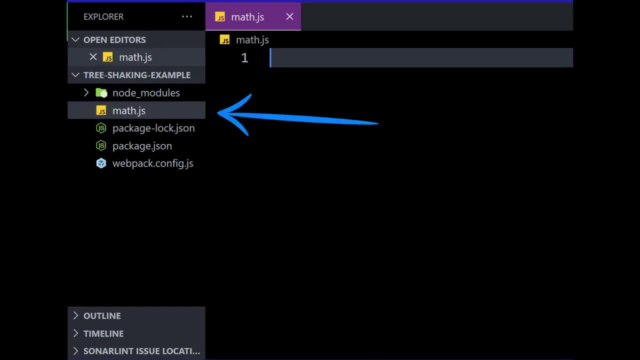 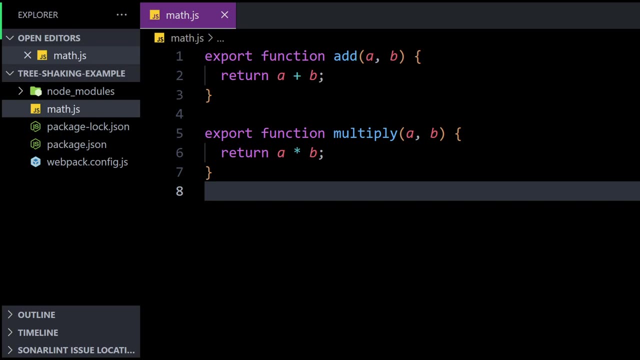 Now create a new file named matjs in the root directory of your project with the following code: To keep things simple, I will use these: add and multiply. After that, create a new file named indexjs in the root directory of your project with the: 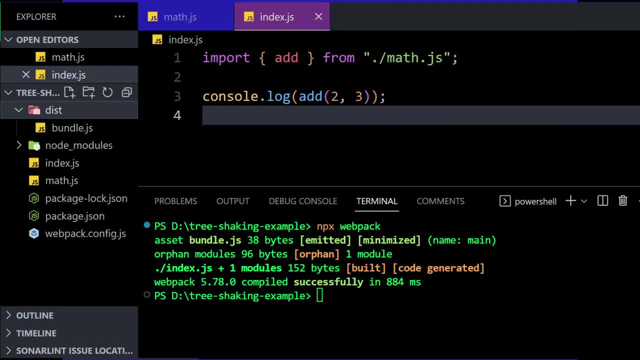 following code. Then run the webpack build command to generate the bundlejs file in the dist directory. This should successfully compile your JavaScript files and generate the bundlejs file in the dist directory. Now create an indexhtml file and add the following code in it: 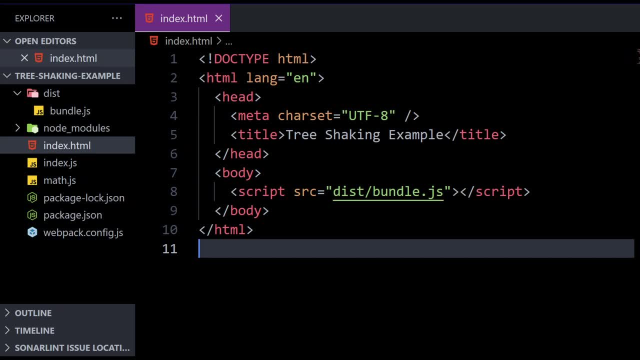 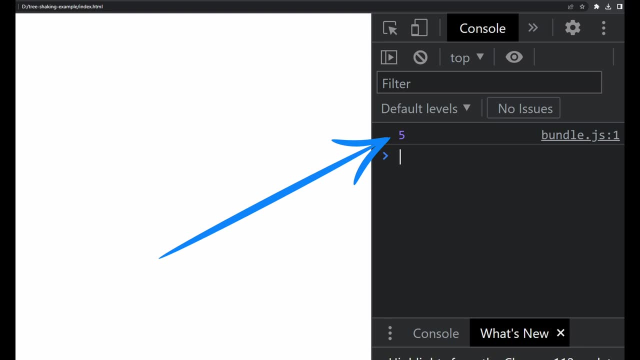 Make sure the script points to the bundlejs file in the dist directory generated from Webpack. Open the indexhtml file in a web browser and check the console log to verify that the add function was successfully imported and used from the matjs module. If the console log is present then it means the bundlejs works fine. 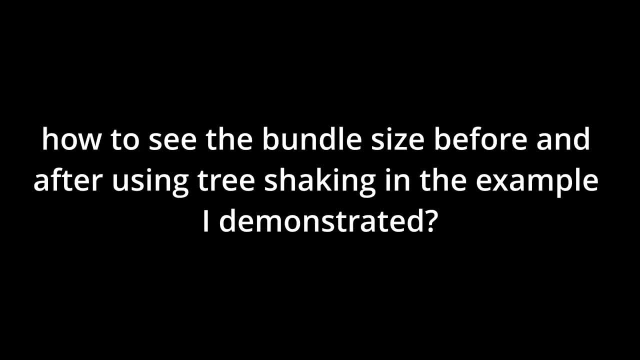 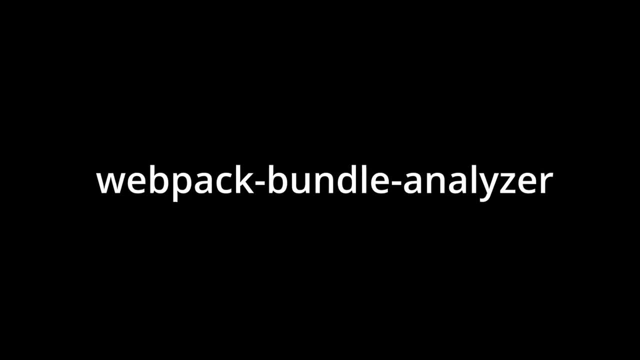 Now how to see the bundle size before and after using tree shaking in the example I demonstrated. For that we can use the webpack bundle analyzer plugin to visualize the size of our bundle and compare the size before and after tree shaking. To install the plugin, run the following command: 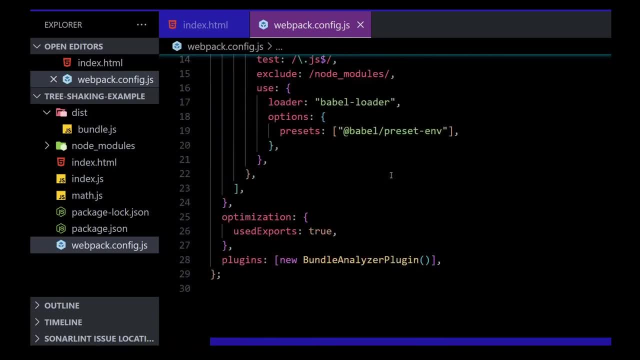 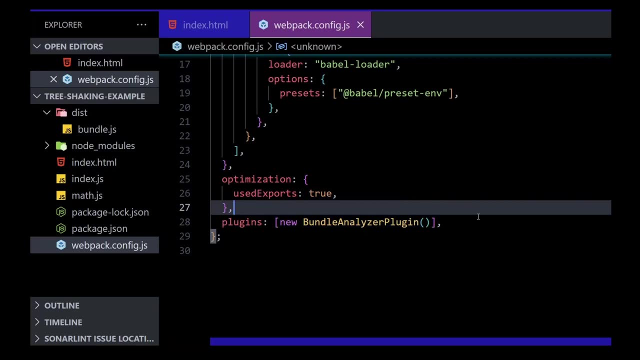 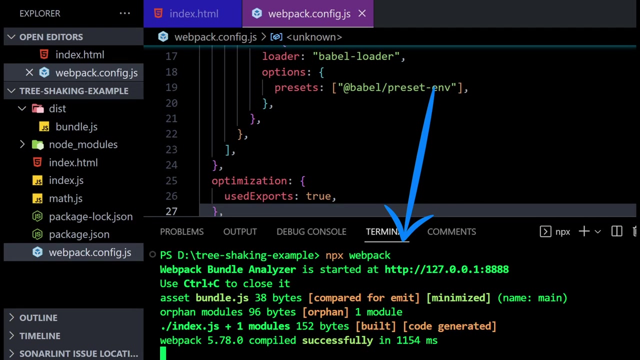 in your project directory. This will add the bundle analyzer plugin to your configuration and generate a report of the bundle size when you run the webpack build command. Now run the webpack build command again. After the build is complete, open the generated report in your web browser. 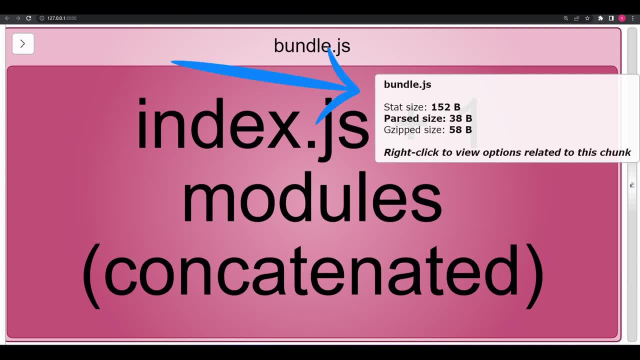 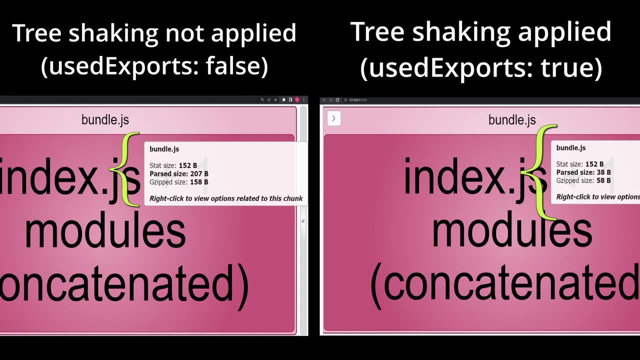 The report will show the size of each module in your bundle and you can compare the size of your bundle before and after tree shaking. You can clearly see the parse size and gzipped size have significantly reduced in the analyzer tool, as well as the size of the bundle after tree shaking is applied. 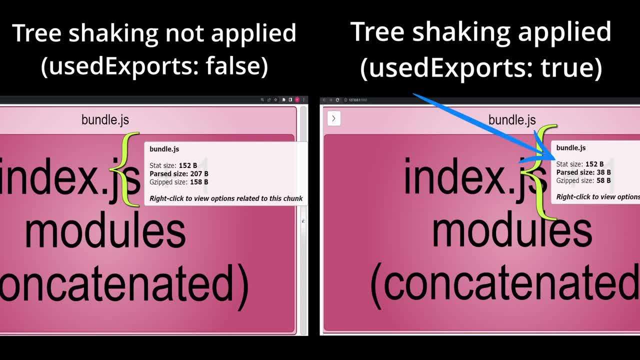 Just to give you an overview of what these terms mean. the stat size is the actual size of the bundle in bytes. It includes the size of all the modules, assets and other files that are included in the bundle. Parsed size is the size of the code after it has been parsed by webpack. This includes 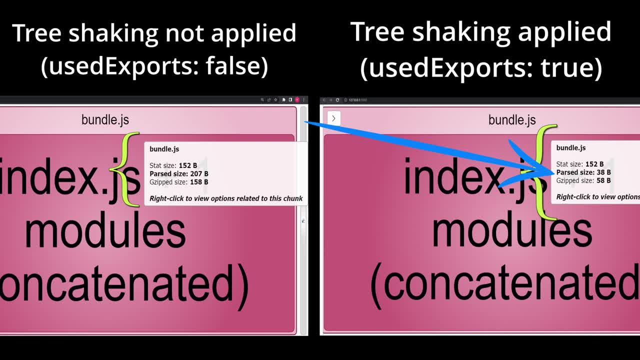 only the code that is actually used by the application and excludes any dead code that has been eliminated by webpack's tree shaking algorithm. Gzip size is the size of the bundle after it has been compressed using the gzip algorithm. This is the size that the bundle will be when it is transferred over the network to the client's. 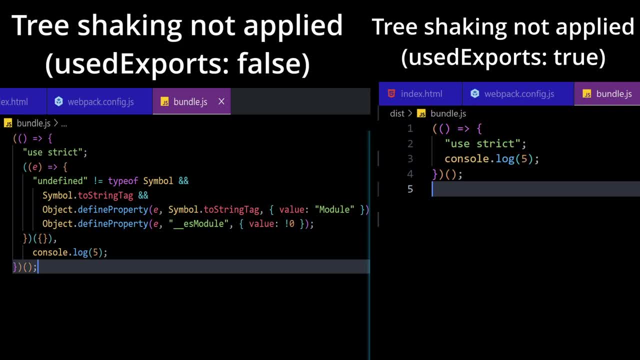 browser. So you can see in the bundlejs file within this directory the contents of the code are significantly reduced before and after applying tree shaking, because it removes all the dead or unused code, such as multiply function and so on. So this is how tree shaking optimizes. 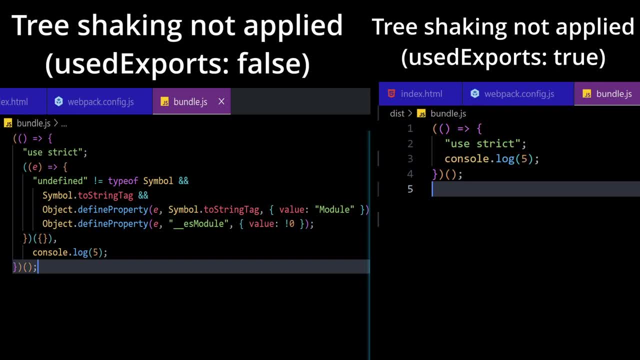 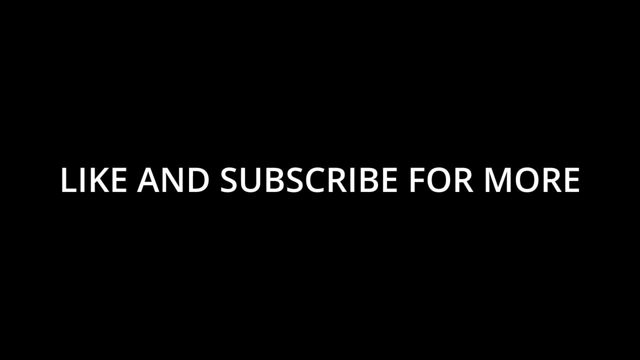 the performance of your application, and I hope you found this example useful. So that's all for the video. If you found this video insightful, then don't forget to like and subscribe and, as usual, stay tuned for more.